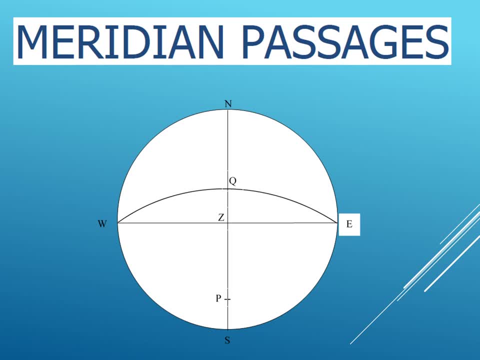 A celestial sphere is a sphere of infinite radius, and that is what is represented by the circle here. It is a sphere of infinite radius. If I look at the celestial sphere from the top, then the observer's position on the celestial sphere is denoted by Z, That is, you in the lens. 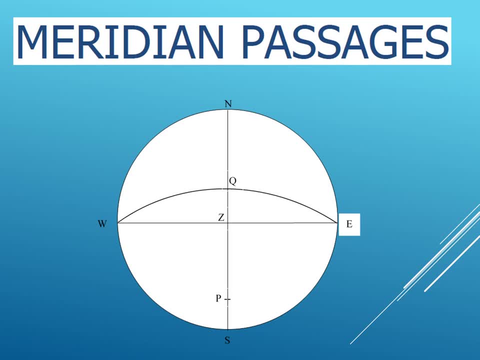 The observer is in the center of the sphere. that's you, Zerber. Zenith stands for Z. Now WQE is the celestial equator or the equinox, all right, equinoxial, rather, not the equinox, the equinoxial. So the celestial equator when projected, when the 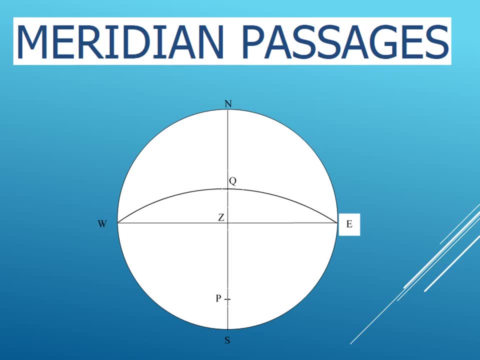 when the earth's equator is projected onto the celestial sphere, it's called the equinoxial or the celestial equator. that is denoted by WQE, So north is denoted by n and south by s, so naturally W and E denote west and east, and each point on this circle is 90 degrees away from the observer. 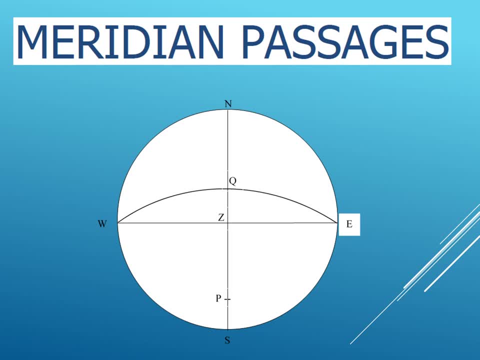 all right, that is observer Zenith. that is Z Now, if you think about it, so far I have not shown you the position of the celestial body. Now the celestial body will rise from the east and set on the west, and it has a transition, so it 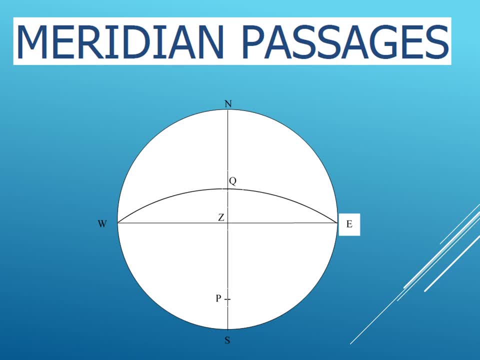 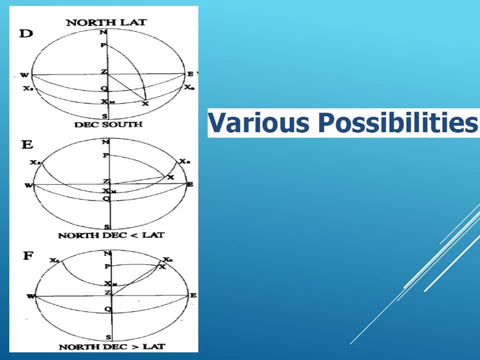 ship. we call it the noon time or the noon passage because it happens very close to 12 o'clock in the afternoon, but it is not exactly at 12 o'clock. it can be a few minutes before, a few minutes after 12 o'clock, but it's still called noon position or rather noon passage, but it's. 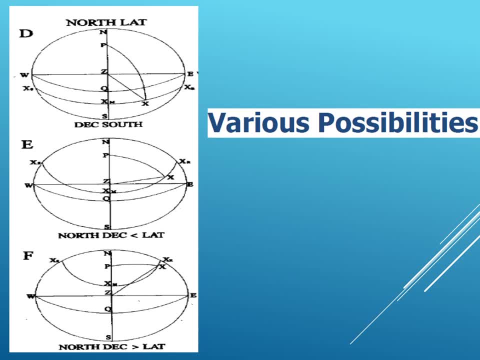 actually, the correct terminology for this is median passage, and the altitude that we obtain at the time of median passage is called the meridian altitude. at this point, the sun is at its highest altitude and it's exactly on the observer's meridian. well, this will, of course, 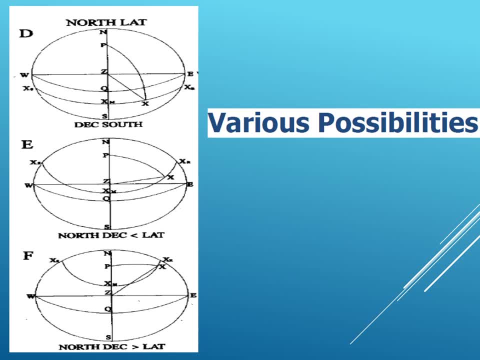 depend on the observer's longitude. but for observers with different longitude, the sun will reach its meridian passage at different points of time. all right, that will depend on the observer's longitude. but for observers with different longitude, the sun will reach its meridian passage at different points of time. all right, that will depend on the observer's. 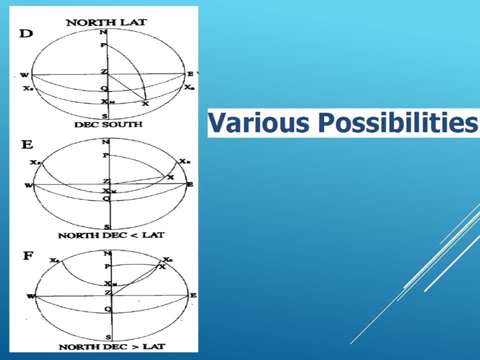 longitude as well. so if you look at the drawings here, there are a few different cases that i've shown you, and if you look at the first case, there it is showing that the latitude of the observer is north latitude. here the celestial equator is denoted again by wqe, that is, the equinoxia. 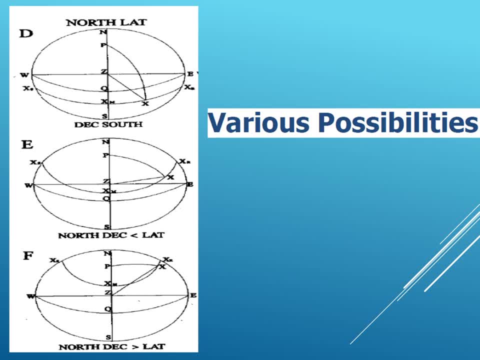 you can see the celestial's body passage denoted by xr on the right and then x on one point of the trance of the transit. xm is the meridian, is the is the point of time when the celestial body has reached its meridian passage. for the 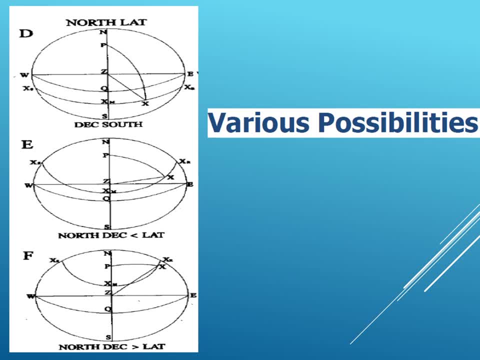 observer z and then xs on the left is the setting of the celestial body. so the celestial body rises from the east, goes through a passage, or goes through a transit passage, and then sets on the west during this point of time, whenever it reaches its maximum altitude with respect to the observer. 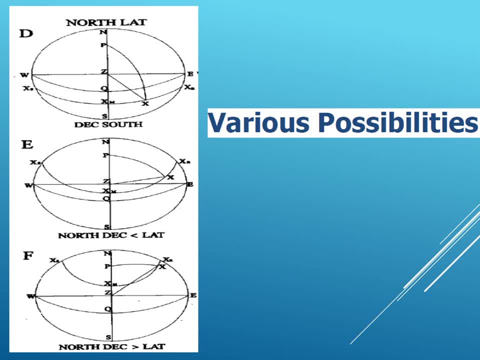 and it is exactly on the observer's meridian. you can see that that is the point of the meridian passage. so in the first example the observer's latitude is north, but the declination of the body or celestial body is south, because, you can see, the passage of the celestial body is 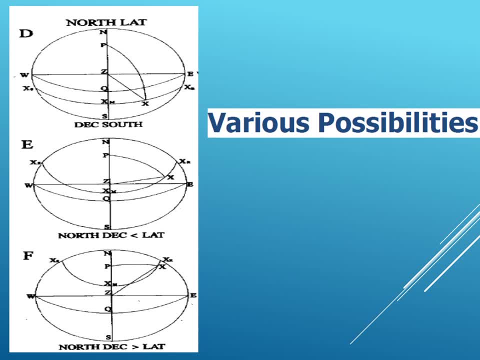 south of the celestial equator, or the equinoxial zx in this case, or in each case, becomes the zenith distance. all right, px is the polar distance. so if you see the second example, then you can see here the body's transit is again from the east. 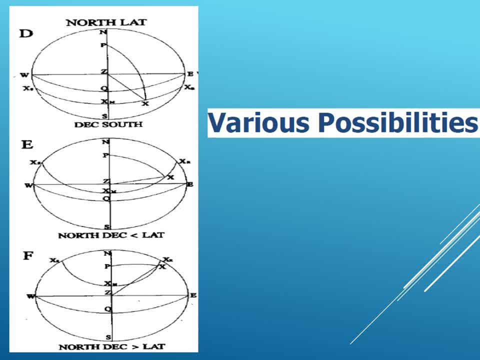 at meridian passage, when it is, reaches its, when it reaches the same median as the observer and then sets on the west. and then it reaches the same meridian as the observer and then sets on the west, but this time the declination of the body is north. 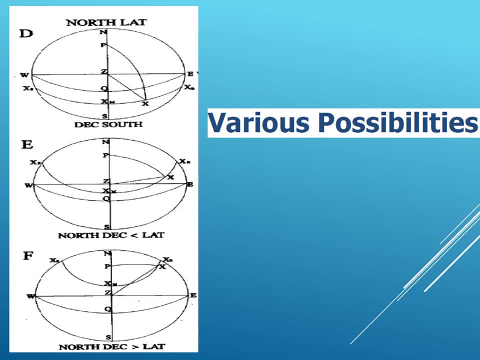 all right. so the declination of the body is north. because the passage of the celestial body is north of the equinoxia zq, is the observer's latitude all right? in this case, again, the observer is also north of the equinoxial, so the observer's latitude is also north, if you can see the distance of. 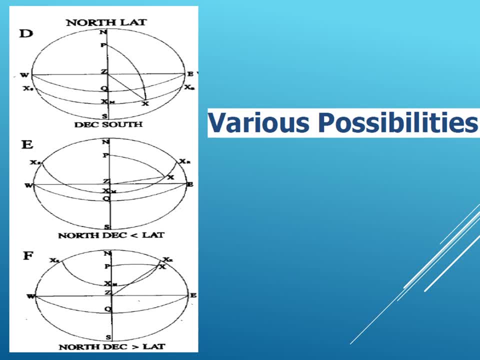 with respect to qx, you will see that zq, or the observer's north latitude, is much greater than the celestial body's declination. all right, so zq denotes the observer's latitude, qx or xq denotes the declination of the body. then we take the third example. in the third example, again, the celestial 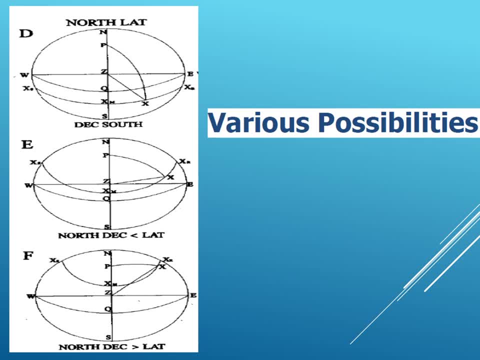 body is also having a north declination and the observer's latitude is also north, because the observer, as well as the celestial body, is north of the equinoctial. in this case, you can see, the distance between xq, which is the declination, is much larger than the observer's latitude, which 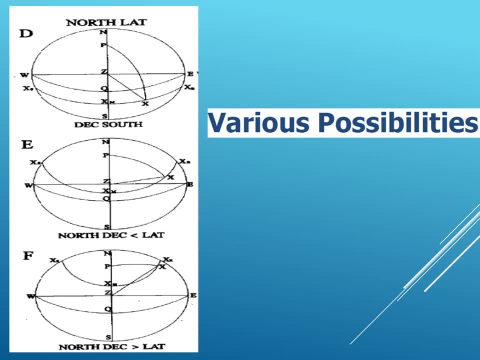 is zq, although both are in the north. all right again, zx becomes the zenith distance. but what you have to note in each of this drawing is that you can see that the meridian passage is occurring in the north of the equinoctial body and the observer's latitude is also north because the 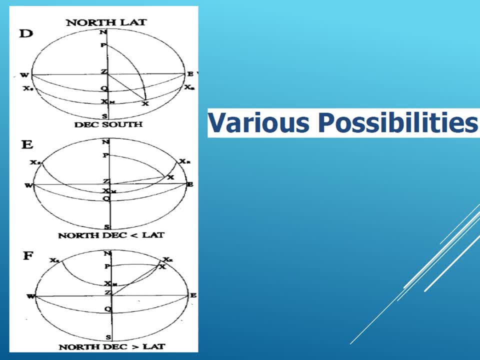 celestial body is on the observer's meridian, so they are all in kind of one vertical line if you look at it from a respect of the celestial sphere. so in the celestial sphere they are all in one vertical line. their meridian or their meridian, celestial meridian, is the same. 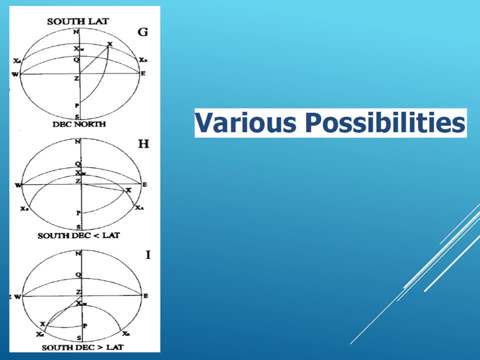 in this case. here i am showing you examples of what happens when the celestial observer's latitude is south. so you can see, here the observer, which is the celestial body, is on the observer's zenith is south of the equinoctial or the celestial equator denoted by wqe. 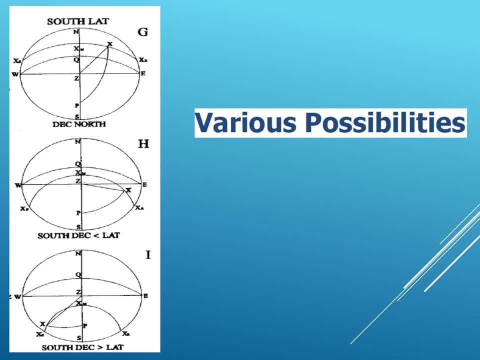 but the declination is north in the first case, right, and then you can see that zq, although the observer's south latitude may be greater than qx, but the latitude is south. so in each of these three cases you can see that the observer is south of the equinoctial. 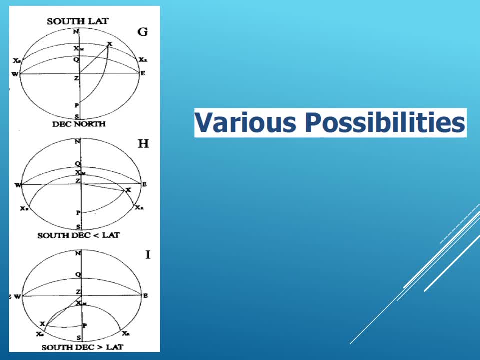 the meridian passage is still occurring when the body is exactly on the observer's celestial meridian, that is xm. body is still rising from east and sitting on the west and you can see here in different cases sometimes the declination is larger than the latitude, sometimes the latitude 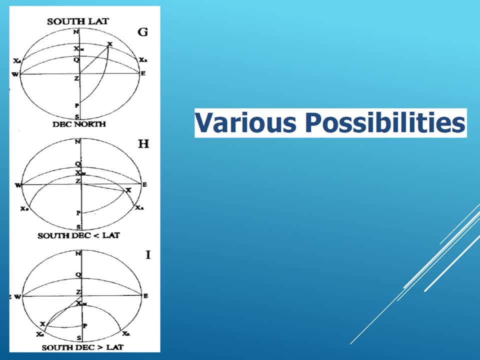 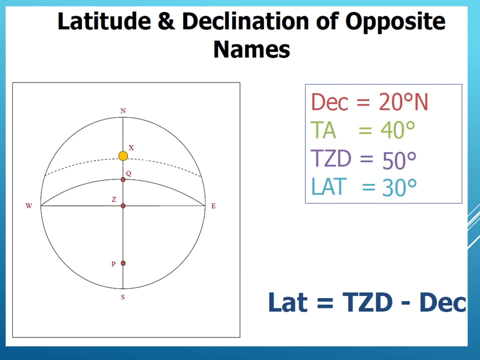 is larger than the declination. but what you have to remember is: zq denotes the observer's latitude and qx denotes the celestial body's declination. all right, so let's take this example here and you can see here, for example, if the declination is 20 degrees. 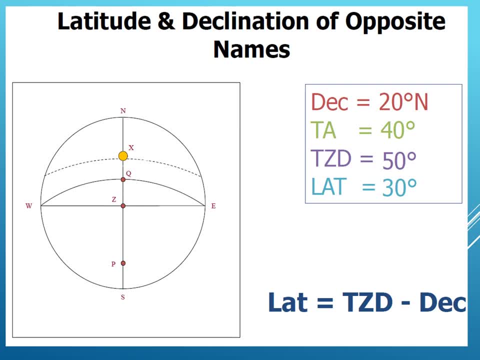 north. that is denoted by qx. so qx is equal to 20 degrees north. so declination of, let's say, the sun is 20 degrees north. here true altitude may be 40 degrees, true zenith distance, which is zx, is 50 degrees. all right, so let's take this example here and you can see here, for example, if the declination 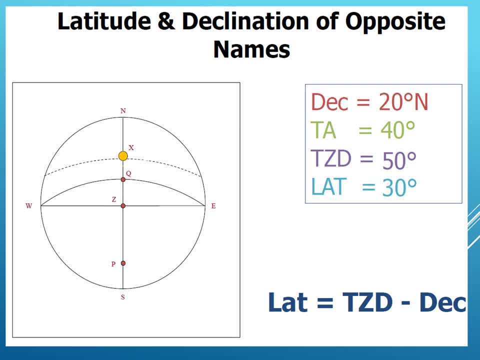 is 20 degrees north. so true zenith distance, which is zx, is 50 degrees. so your latitude will be 50 degrees, that is true. and distance minus the declination, which is qx, 20 degrees and equal to latitude, will be 30 degrees. so zx is a zenith distance which is 50 degrees. qx is the declination. 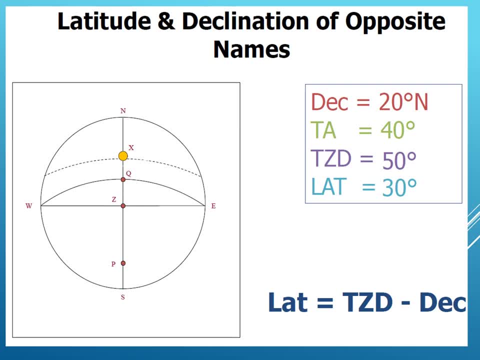 which is 20 degrees. so your latitude, which is denoted by zq, will be 50 minus 20 in this case, which is 30 degrees. now can you tell me what is the latitude here? is it north or south? so you can tell me that, if you look at the celestial equator, which is denoted by the wqe. 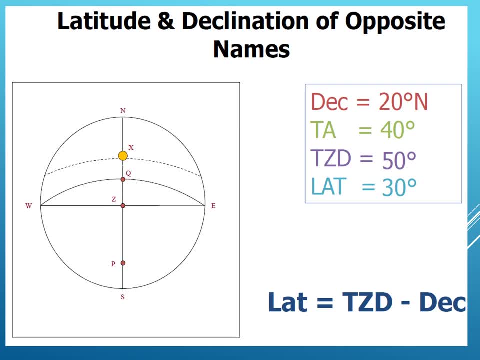 it's also called the equinoxial. so look at the observer's position with respect to the equinoxial. is the observer south of the equinoxial or north of the equinoxial? so you can see the observer is south of the equinoxial, which makes our latitude south. so 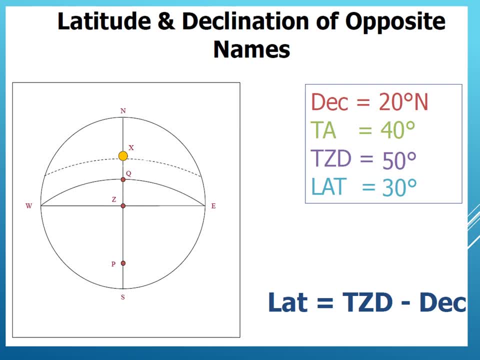 it is 30 degrees south. what about the declination of the body? you can see the declination body is north because the body or the celestial body x, denoted by x, is south of the equinoxial. so you can see that the observer is south of the equinoxial. 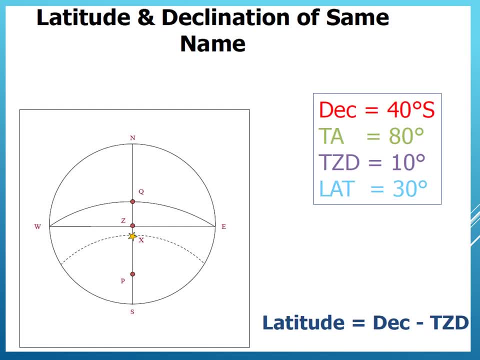 north of the equinoctial, In this case. here you can see that the declination is south, because the celestial body is south of the equinoctial. In this case declination is 40 degrees south, Assume that the true zener distance, or zx, is 10 degrees. So in this case, 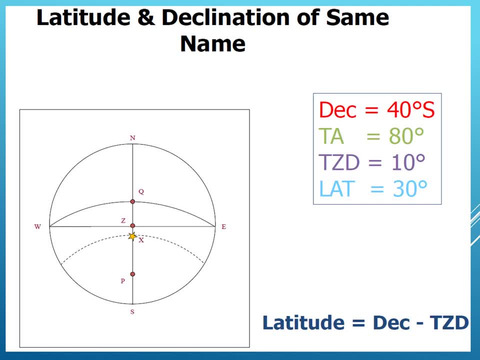 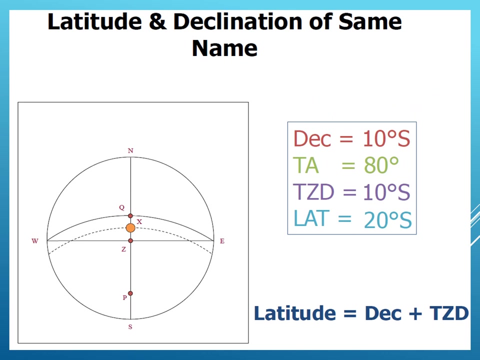 the latitude, which is zq, becomes declination, which is qx minus zx, which is zener distance. In this case latitude is 30 degrees and again latitude is south because the observer is south of the equinoctial. The third example: as you can see, the declination is again south, The celestial body is south of. 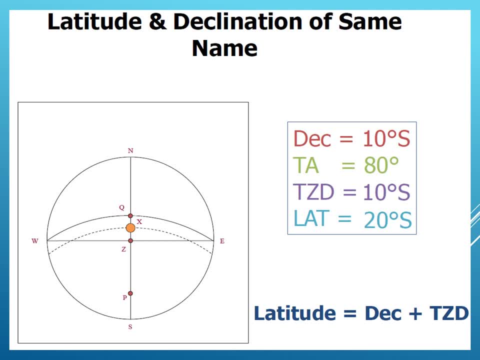 the equinoctial. In this case let's say qx, which denotes the declination- is 10 degrees south. true altitude is 80 degrees. true zenith distance is 10 degrees south, so zx is 10 degrees south. so your latitude will be zx plus qx, which 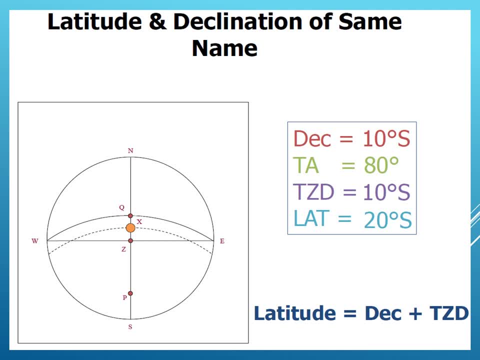 is 10 plus 10 equals to 20 degrees. the observer is still south of the equinoctial and that is why your latitude is south. all right, so zx will be the zenith distance, all right. so these were some few different examples. like i told you, each point on the rational horizon is 90 degrees away from. 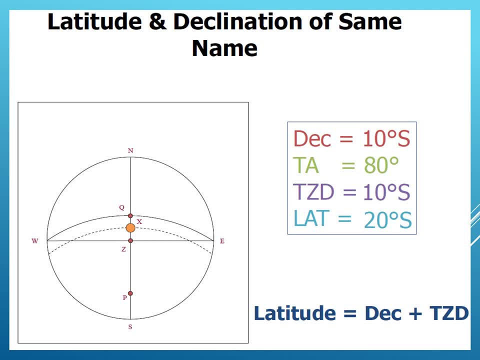 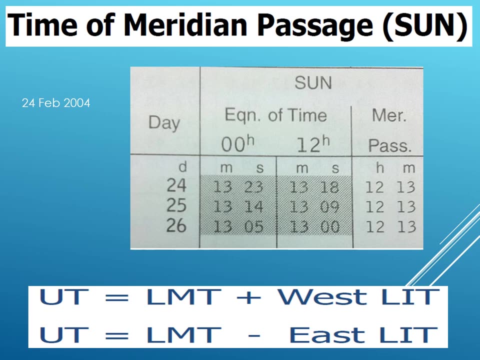 the observer zenith. if zx is the zenith distance, then the distance of the x from the each point on the celestial or the rational horizon becomes the true altitude. in that case, all right. this here is basically showing you that the time of the meridian passage can be obtained from the nautical 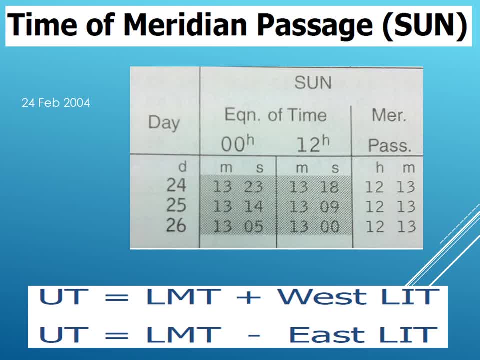 almanac. so i have covered all this in my numerical examples but just i'm showing you here- if this is the first video you're watching- that if you go into the nautical almanac and if you look on the right side of the nautical almanac and bottom, bottom of the right hand side of the nautical